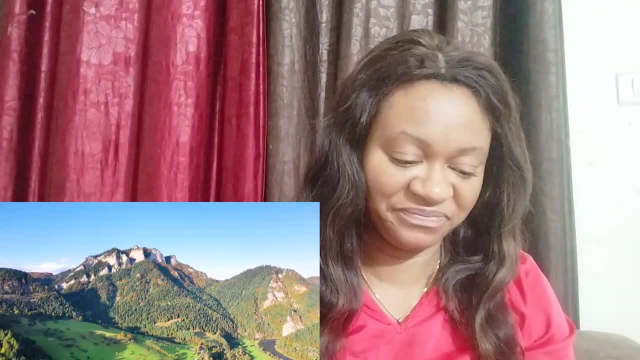 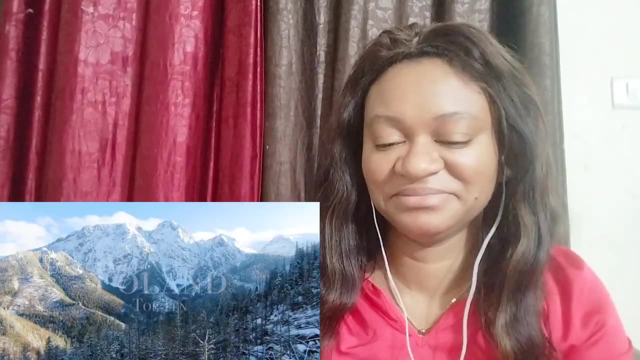 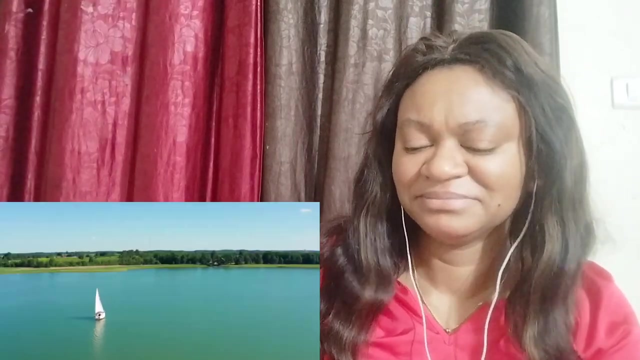 guys. what's up, guys? my name is ryan and i want to show you some of my top 10 places to visit in poland, my favorite places in the enchanting country of poland. so here is my polish top 10.. poland is home to some of the world's most stunning landscapes, from the medieval old town of gdansk to 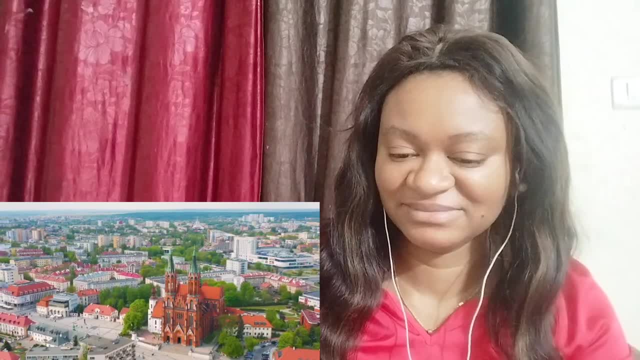 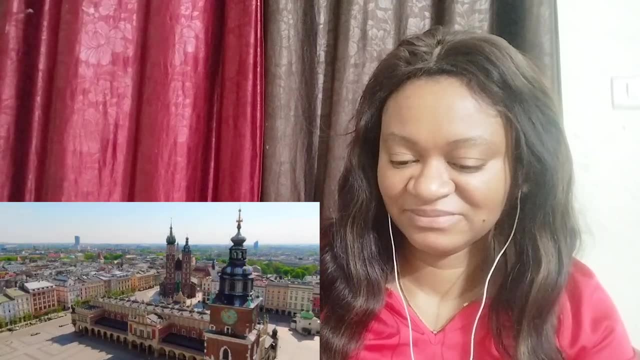 the towering tatra mountains. poland has so much to offer. let's start this video off at the impressive city of krakow. now, this may be one of my favorite cities in all of poland, located in the southern part of the country, but it's not the only place to visit in poland: it's also the most beautiful. 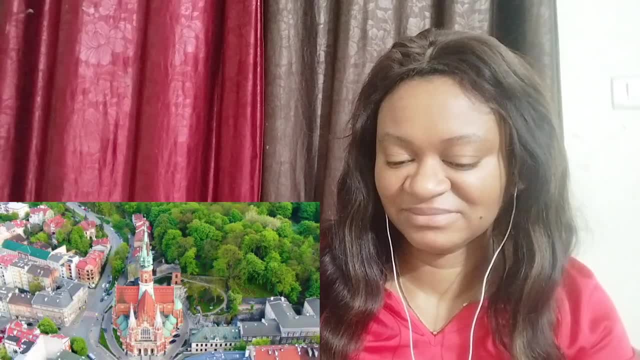 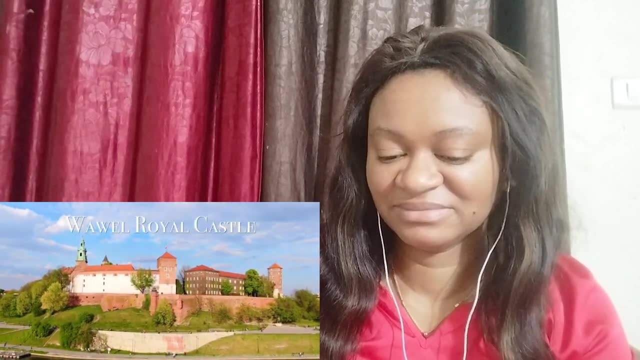 city in the entire world in the 17th century. krakow was founded all the way back in the 7th century, so you best believe it's full of beautiful history and architecture now. one of the most impressive site is the wowell royal castle. it was built during the 14th century and was the first unesco. 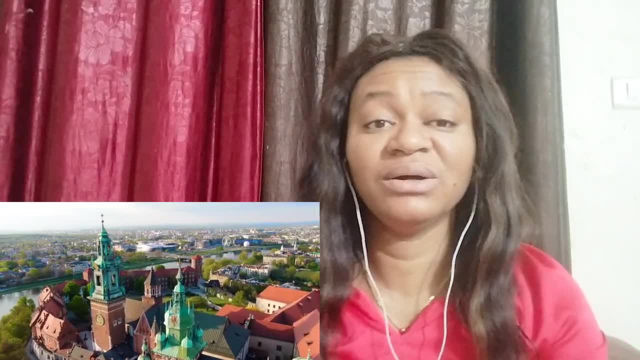 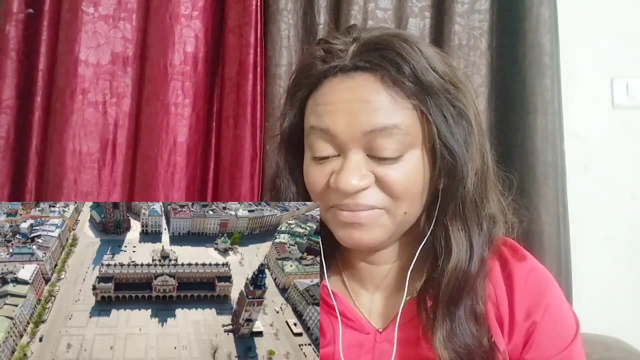 ruled heritage site. it features architectural styles from the medieval, renaissance and baroque periods. now, from the castle, you can make this short 10 minute walk to the main square. this dates all the way back to the 13th century and it was the largest medieval town in squares. 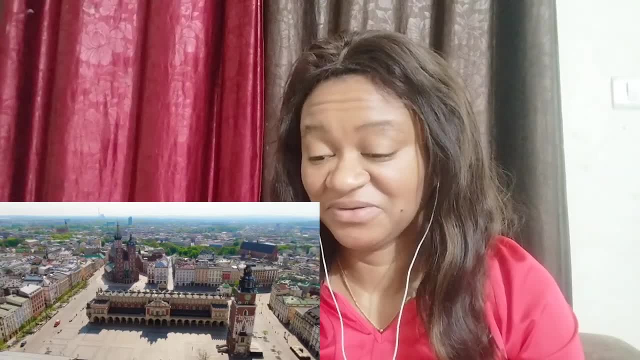 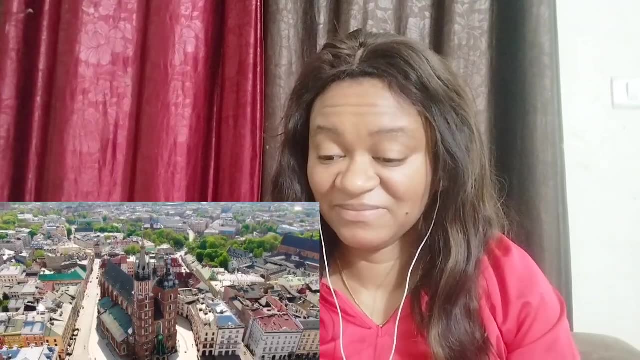 in all of europe, which is pretty crazy, and it's just fascinating to think of all the history that took place here. now, in the corner of the square is the saint mary's basilica, which was built back in the 14th century, and it's a perfect example of polish gothic architecture. another interesting feature of krakow is the kościuszko mound. it's an artificial hill that was modeled after other prehistoric mounds in the city. it was built in 1823 to commemorate the national hero named tadeusz kociuszko, the the mount here is the hardest mountain in the city in the history of poland, and the population is 10 to 100 million people, so that's a lot to consider. 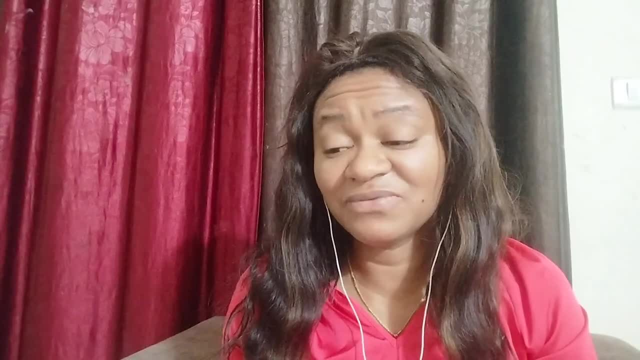 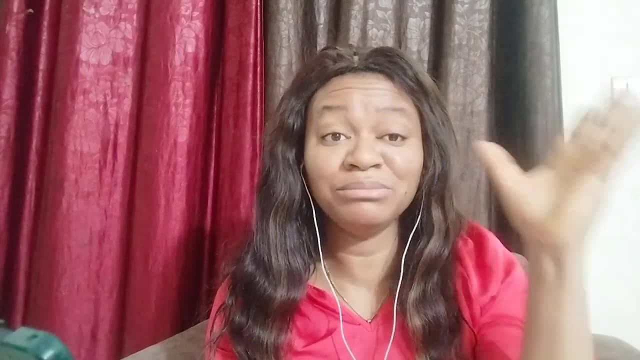 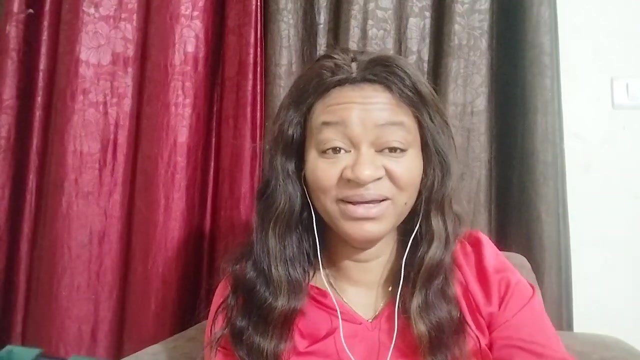 the mount is 112 feet. Wow, I really love this place. Artificial mountain Sounds so good, guys. Imagine seeing artificial mountain in the middle of a city. This is a magnificent country, guys. Awesome people, Let's continue, guys. And there's a serpentine path that takes you to the top, to. 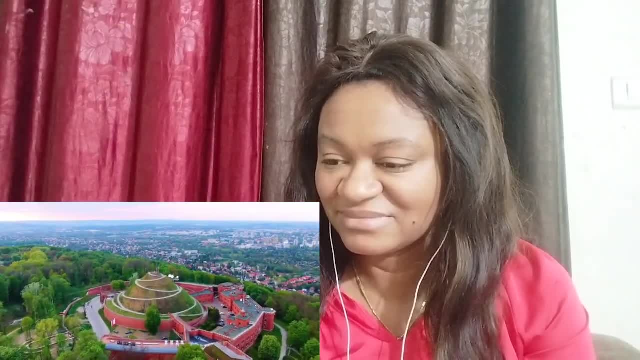 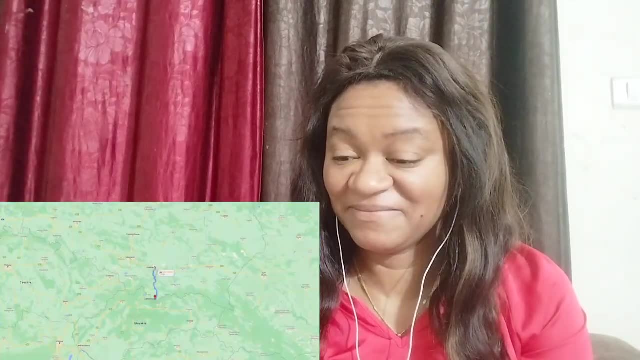 enjoy the panoramic views of Krakow and the Vistula River. Krakow is just such an amazing city and I hope you all can visit. After Krakow, we're going to head to the Tatra Mountains, Now located about two hours drive from Krakow. the Tatras are a stunning mountain range that straddles the Polish 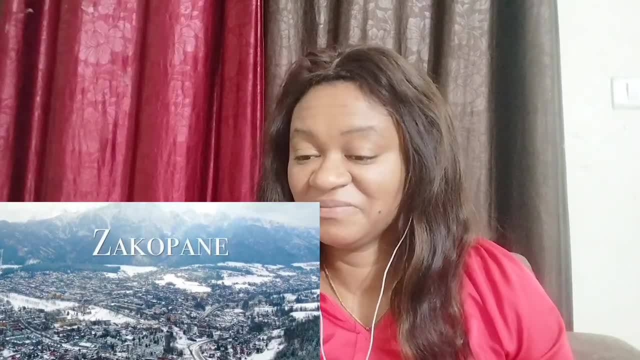 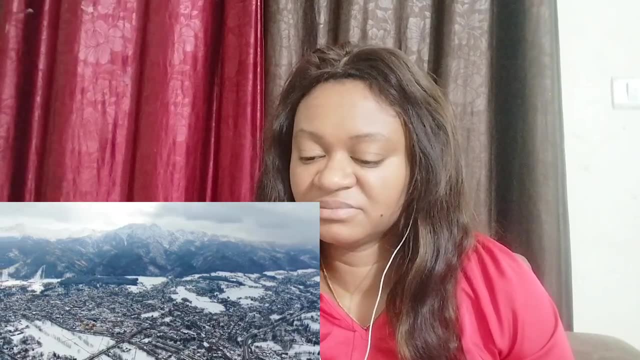 and Slovakian border. Now, the best town to access the Tatras is Zakopane. Now located right at the base of the mountains, Zakopane is the perfect starting place for your mountain adventures. During the wintertime, Zakopane is an ideal place to go skiing, and in the summer months it's a 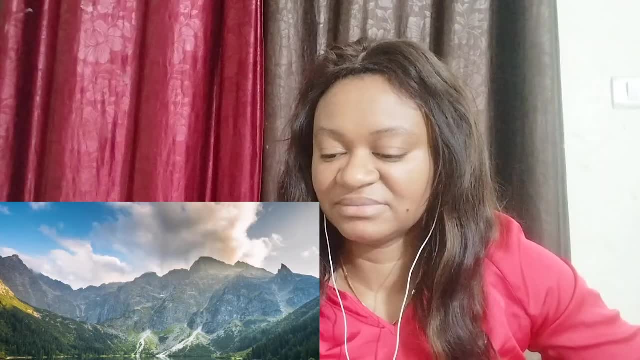 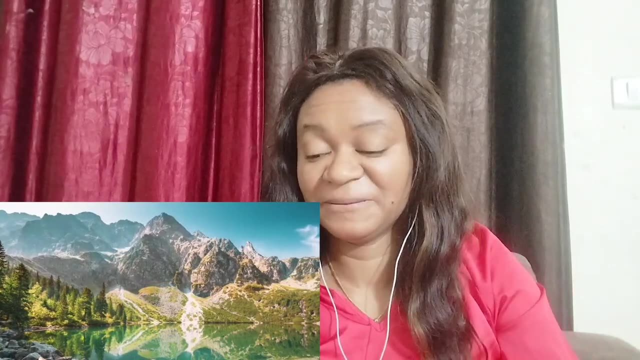 prime place to start your hike into the mountains. One of the most impressive spots in the Tatras is the Morski Oko Lake. You can make the 16-kilometer round-trip trek to the scenic lake. I mean just such a phenomenal view up there. An interesting fact is that the Tatras are the 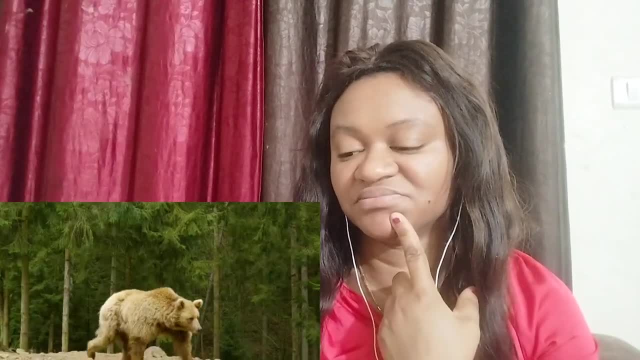 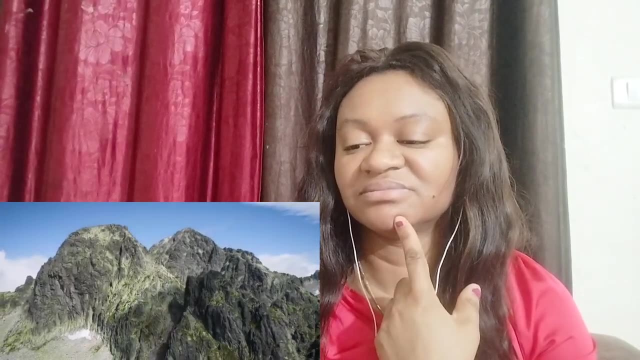 smallest alpine mountain range in all Europe, and they're home to plenty of wildlife, such as the Eurasian brown bear. I just love how the Tatras look. They have such a unique and jagged look to them and I just want to go hiking them this summer. Now, if you're into World War II history. 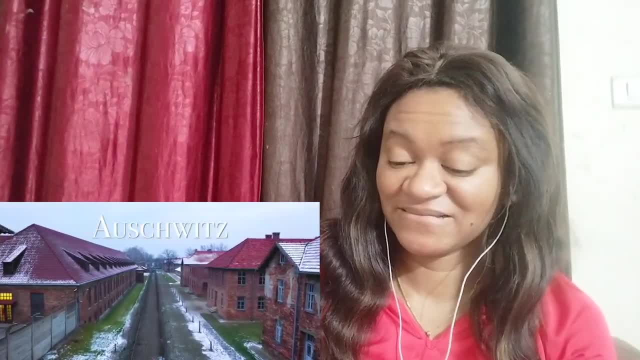 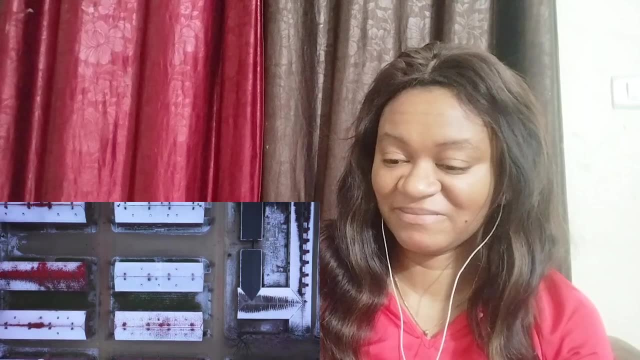 you can visit the Memorial of Auschwitz Concentration Camps. This is located about an hour's drive from Krakow. Now, Auschwitz is infamously known to be one of the most horrific Nazi concentration camps. Over 1.1 million people died here. One of my favorite books I've ever read. 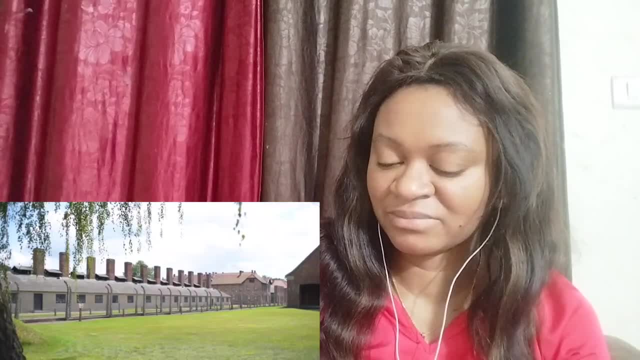 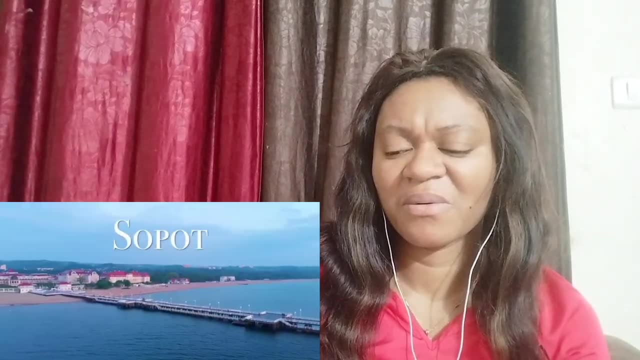 is called The Auschwitz Escape, and it tells the story of how two prisoners made their daring escape from this concentration camp. Now, after, we're going to head to the northern part of Poland to visit Sopot, Now located right on the Baltic Sea, Sopot was established in the 8th century and grew 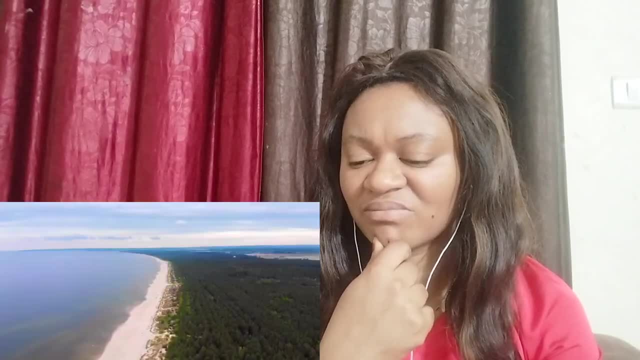 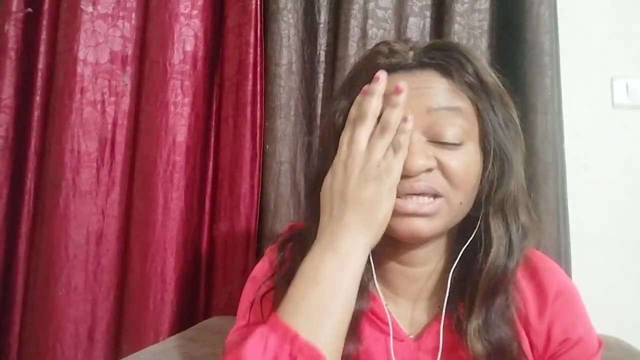 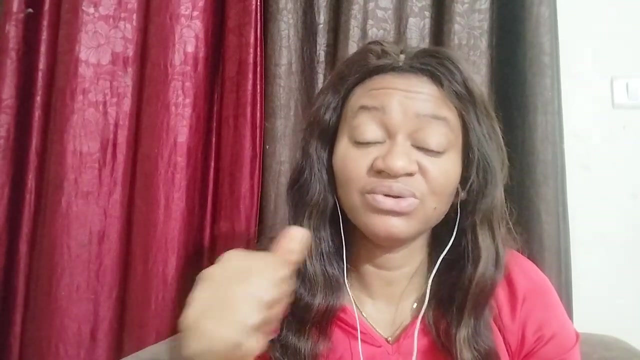 as a commercial trading post and fishing village. Over the centuries, Sopot faced adversity as it was abandoned, burned and then rebuilt. So you guys, I just wanted to say, after watching the war, not the war, I think, before their coronation or before they got independent- become free. 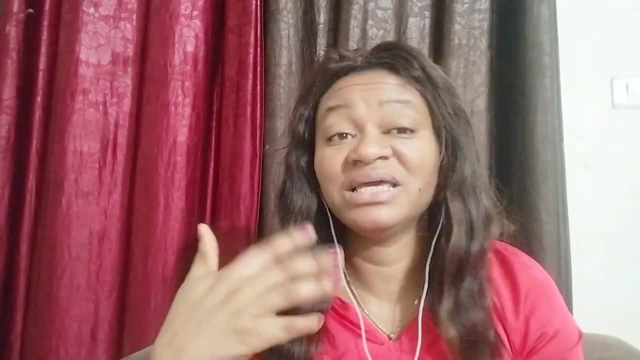 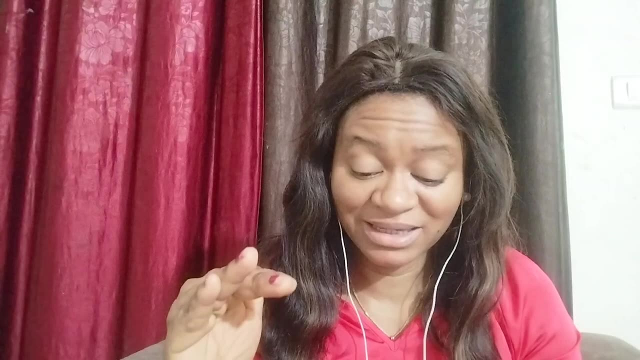 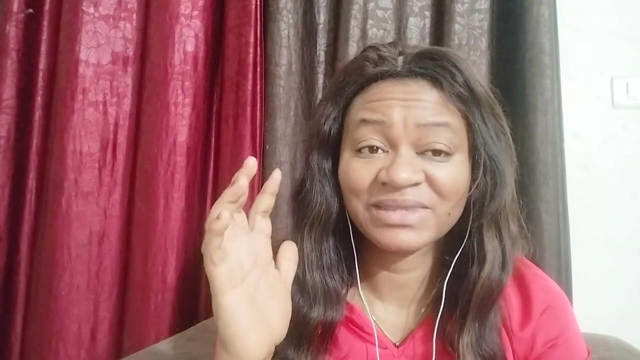 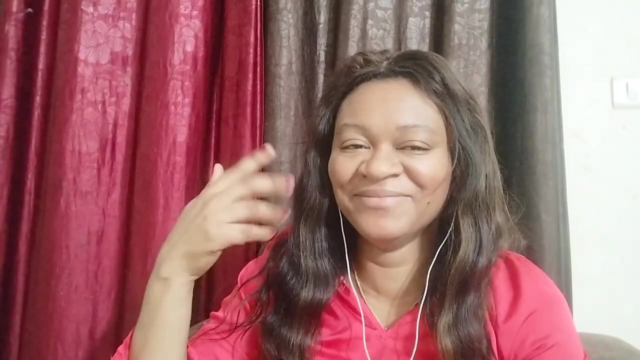 I watched that. I made a video about their animated history and we didn't look how beautiful. it looks like nothing happens there. This is a unique country, guys. This is a beautiful country. The land is blessed. really, Watching it from here, it's beginning to ring in my brain, in my mind, as a bucket list. This is so. 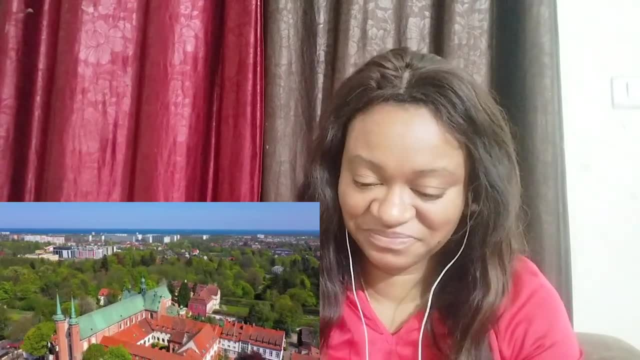 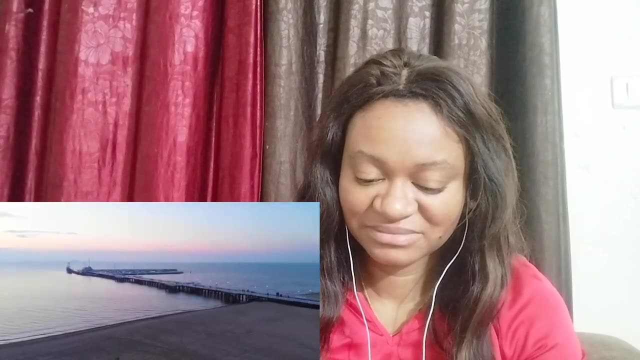 beautiful. Let's continue. In the 8th century, Sopot started to gain popularity thanks to its spa and public baths, and it quickly became a holiday resort town. Today, Sopot is a thriving tourist attraction. While you're there, you can take a walk on your own. You can also go to Sopot's 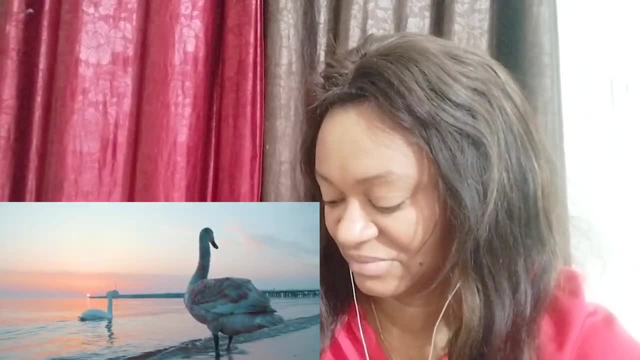 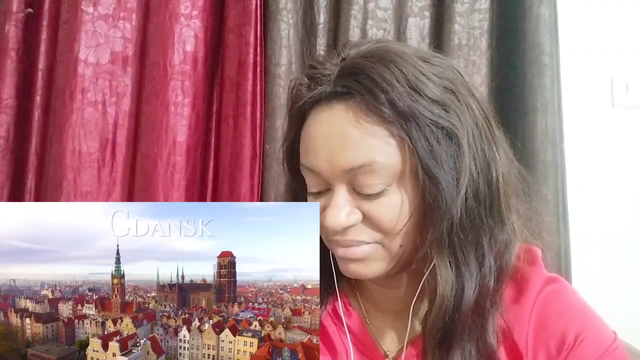 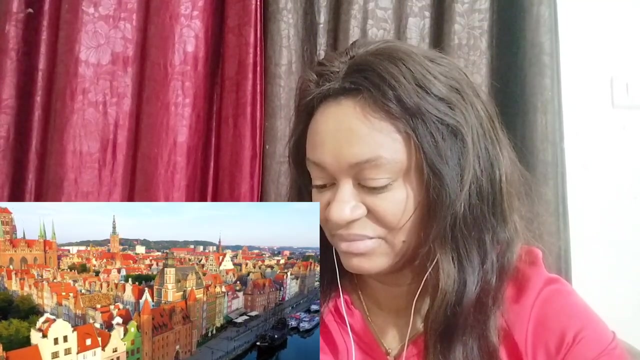 Europe's longest wooden pier, or you can enjoy the swans and endless sandy coastline. Now I understand why it's called the Polish Riviera. Now, after Sopot, we're going to head over to the neighboring Gdansk. Located just a 15-minute drive from Sopot, Gdansk is one of Poland's oldest cities, with a 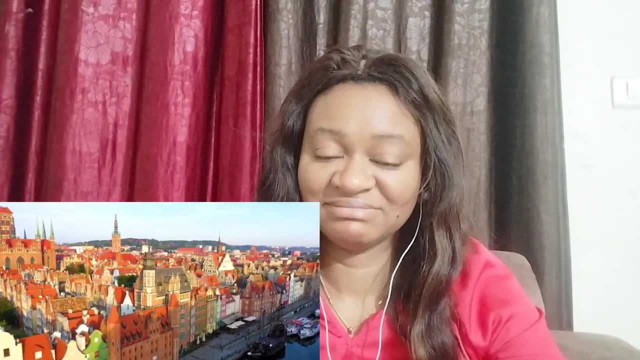 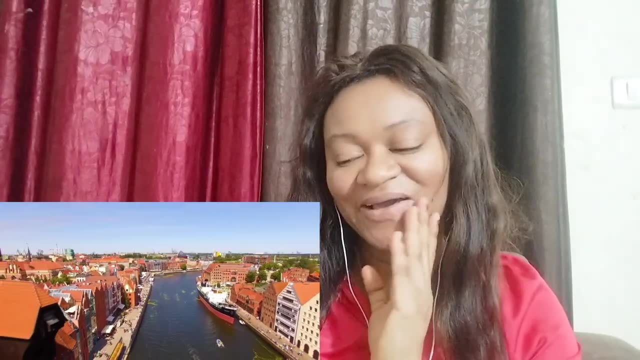 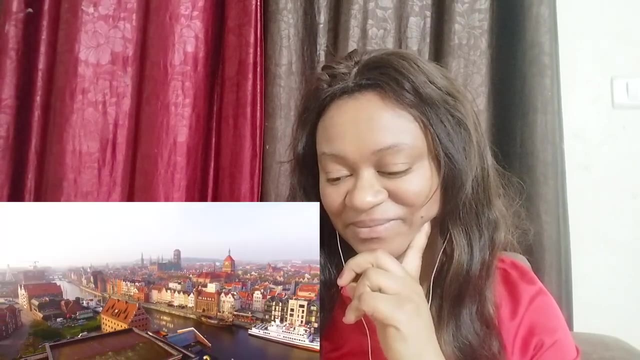 fascinating history with periods of Polish Prussian and German rule. The earliest mention of Gdansk was in the year 997 AD, and during the Middle Ages Gdansk grew as an important seaport. It rose to be one of the wealthiest and largest cities in Poland, until Warsaw's rapid growth in 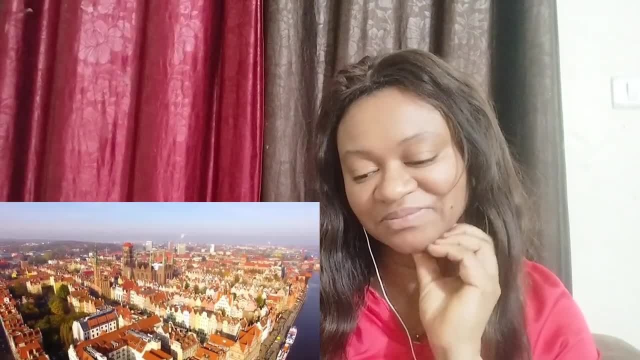 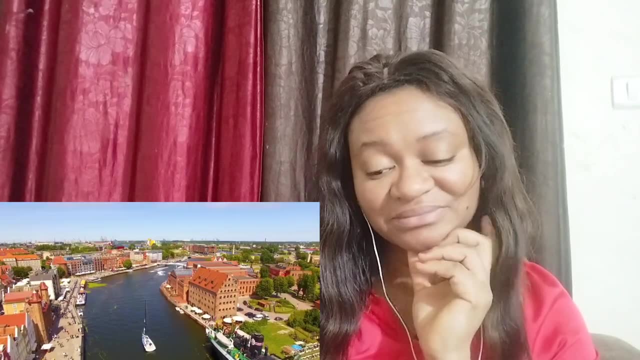 the 18th century. Today, Gdansk is one of Poland's most beautiful cities. I mean, I just can't believe it's old town. It's full of these perfectly placed houses that seem to go on forever. Another really cool feature that I like about Gdansk is how the canal runs right along the old town. It's often 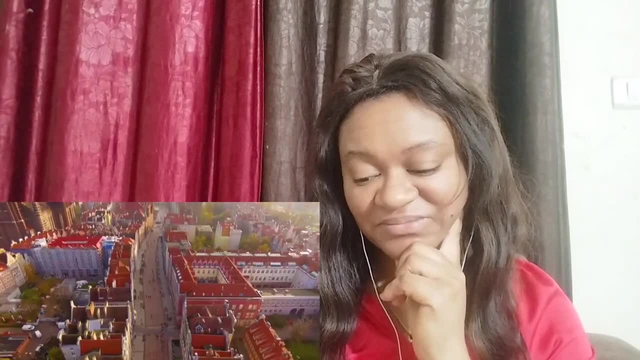 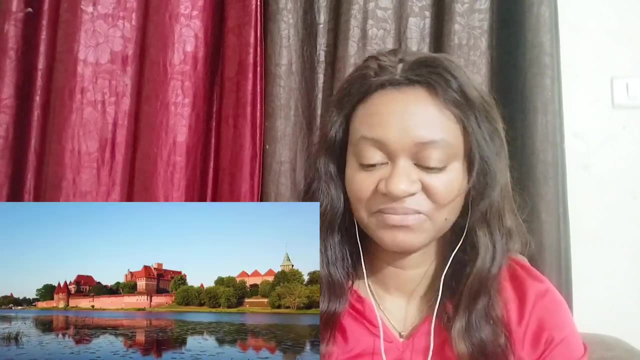 full of ships, and it gives the city such a fun vibe. While you're there, you can just explore the streets of old town or take a walk along the canal. I'm sure you'll love it. Let's go. Gdansk is such an incredible city. Now, just an hour's drive from Gdansk is the Malborka. 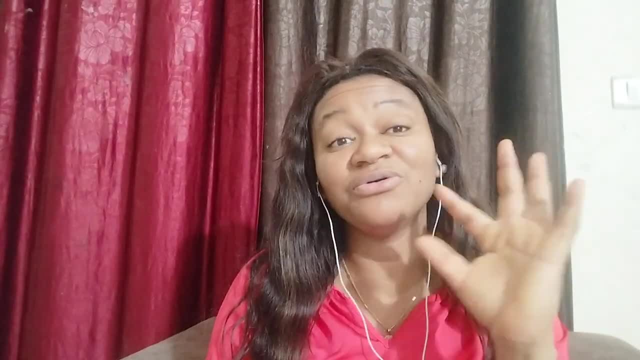 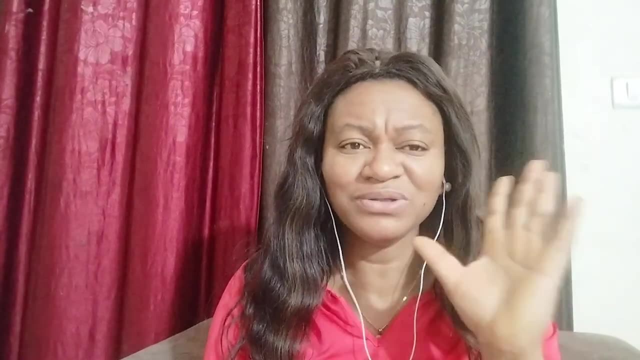 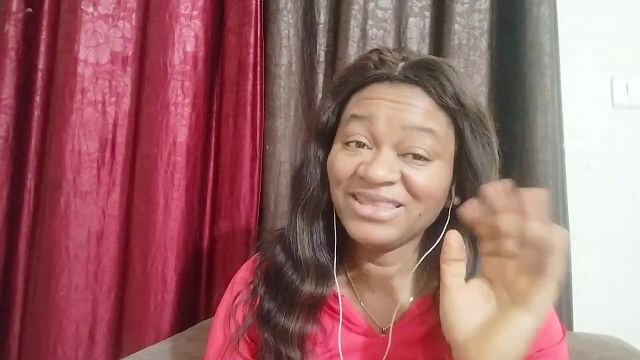 You guys this place. I love the color of the buildings. I just love how they mix it- red, orange, like the way they put the colors make it so colorful and so beautiful. Poland is really beautiful guys. Tell me in the comment section: have you visited Poland or? 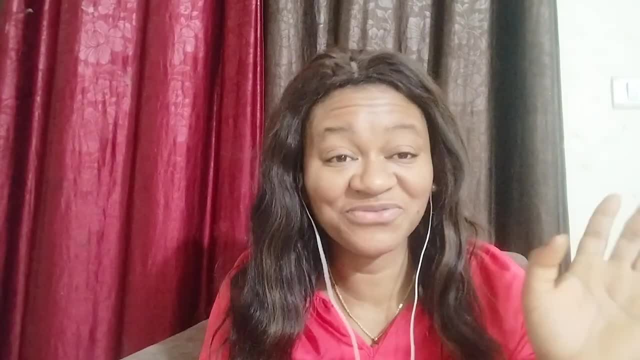 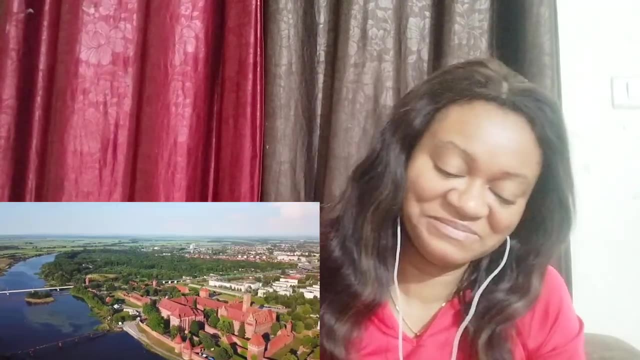 are you from Poland or do you have plans of visiting Poland? Because, if I have my way, I would love to visit Poland. Let's continue, guys. And this is the largest castle in the world by land area, which is pretty crazy. It was. 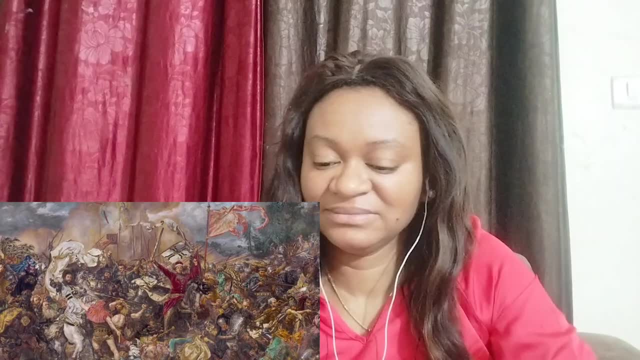 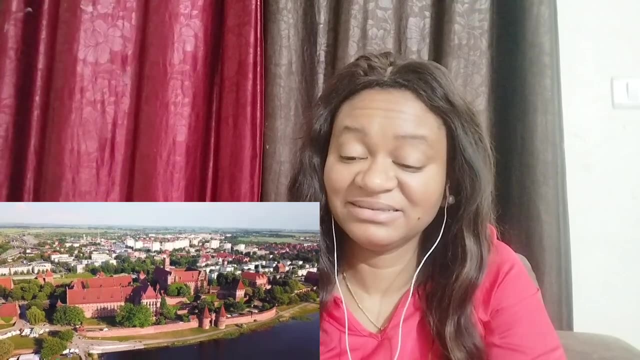 built in the 13th century by the Teutonic Knights, who were German Catholic crusaders. And as the number of the Knights grew, so did the castle, which enclosed an area of 52 acres. I was just crazy to think that people were able to build such buildings back then. 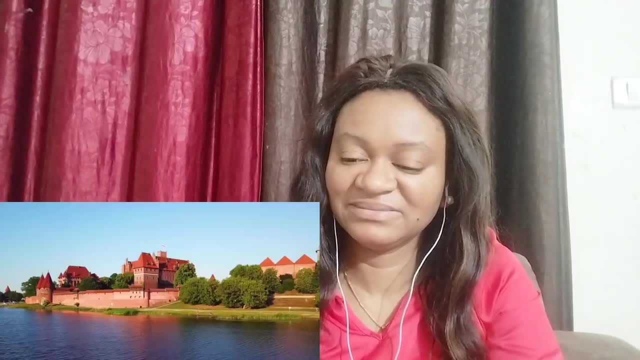 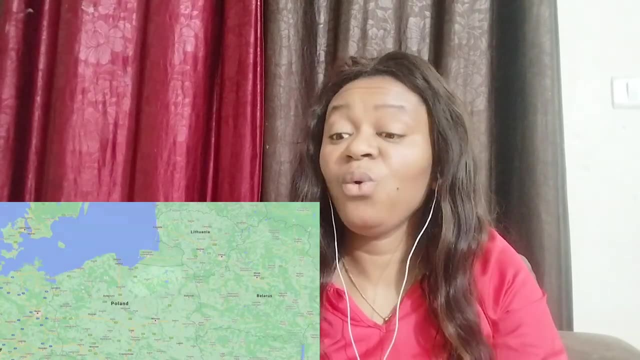 More than half of Malbork Castle was destroyed during World War II, but thankfully it was rebuilt to its former glory. Crazy. After Malbork, we're going to head over to the Missourian Lake District. located in northeastern Poland on the border of Kaliningrad, This lake district is one of the most visited lake. 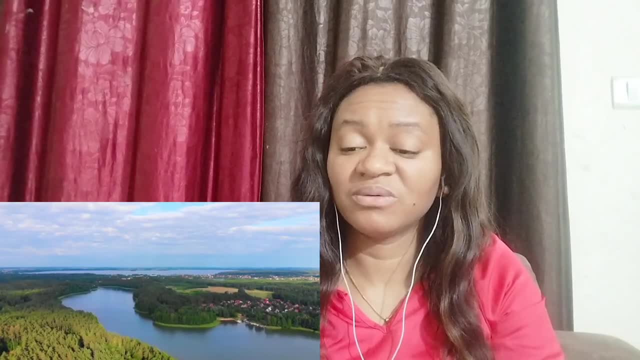 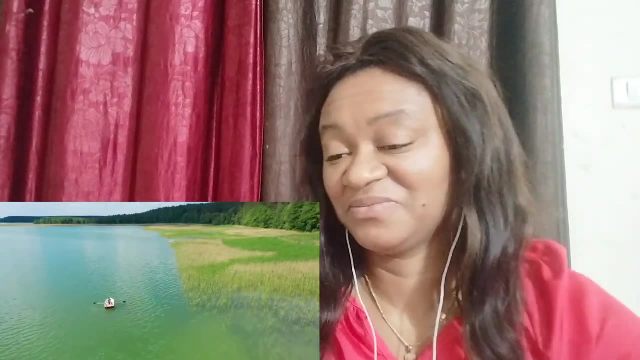 districts in all of Central Europe and it's home to over 2,000 lakes. It's a perfect place to go sailing, fishing or just swim in the lake. I mean, I just can't think of a better place to go on a hot summer day. Now, aside from the lakes, the area is full of beautiful. 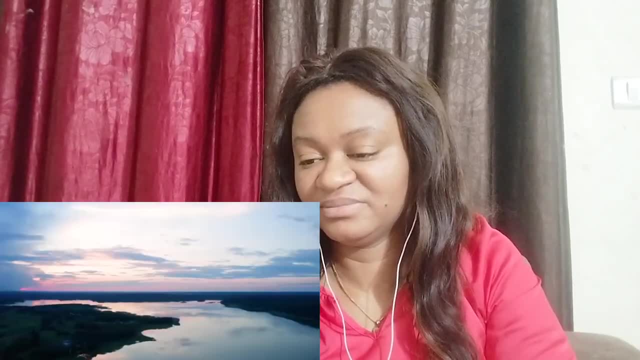 forest, perfect for hiking and exploring. The Missourian Lake District is definitely a hidden gem that deserves to be explored. Wow, this lake is beautiful. I mean, I just can't think of a better place to go on a hot summer day Now, aside from 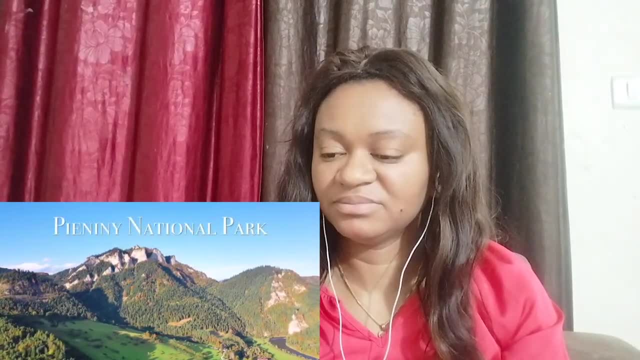 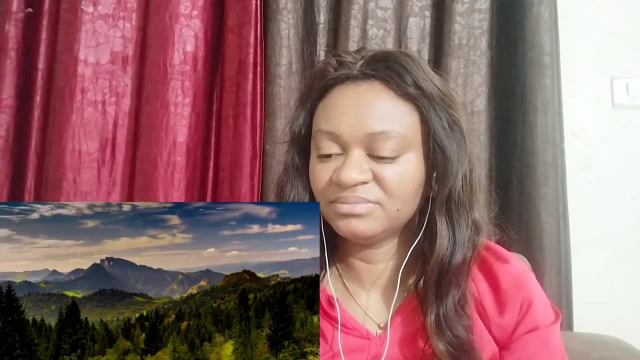 the lakes. the area is full of beautiful forest, perfect for hiking and exploring. Another scenic place for nature lovers is the Pianiny National Park, Now located in both southern Poland and northern Slovakia. Pianiny is one of the oldest and smallest national 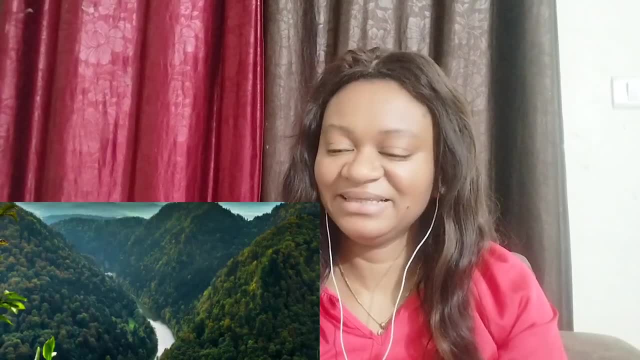 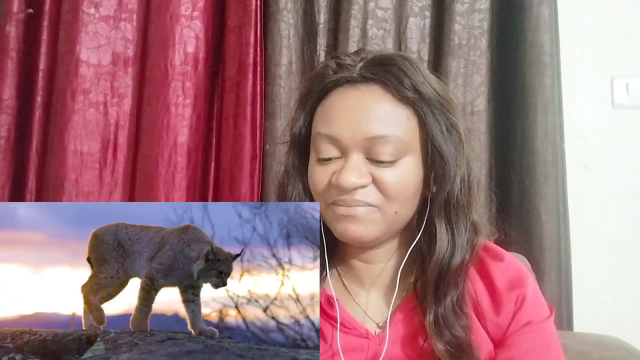 parks in all of Poland. I mean, I just think it's such a beautiful area, The river runs right through it and it acts as a natural border between Poland and Slovakia. The national park is home to many animal species, such as the Eurasian lynx, which I think is like. 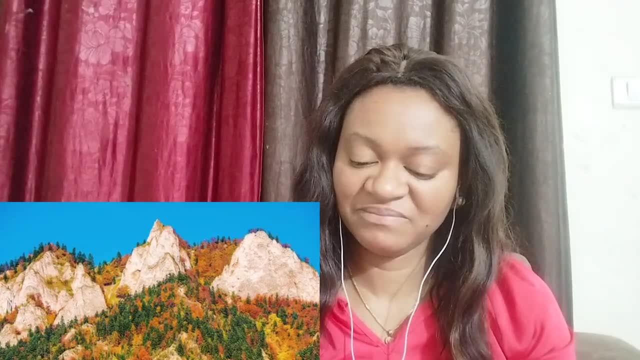 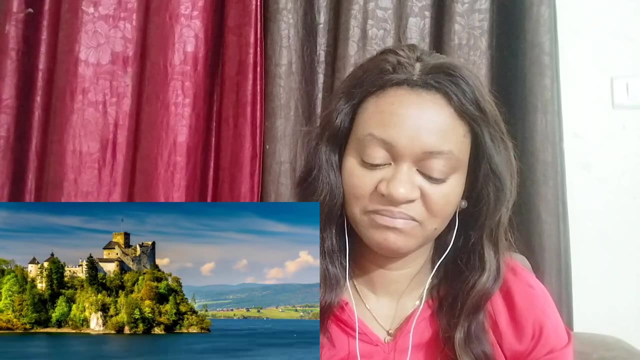 one of the coolest animals ever. One of my favorite features of the park is the three crowns. The rock feature is made up of five sharp limestone peaks that create quite the sight. Now another beautiful nearby spot is the Nijadica Castle This 14th century. 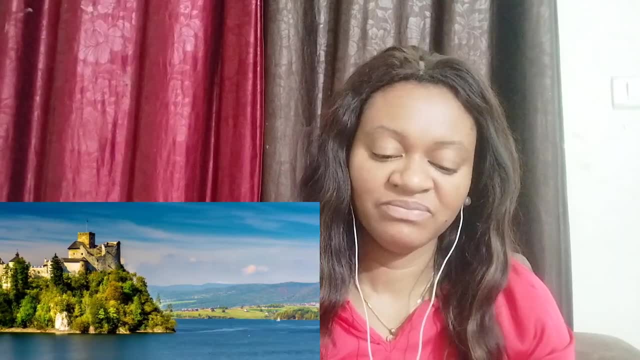 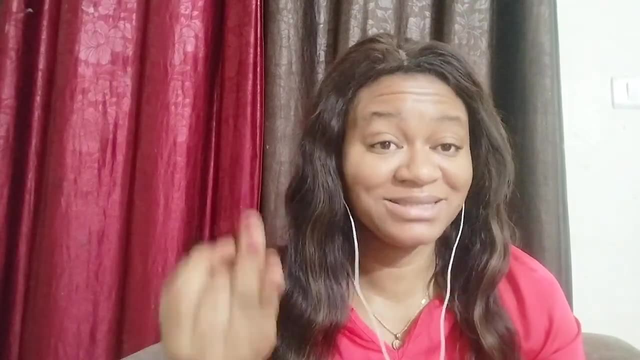 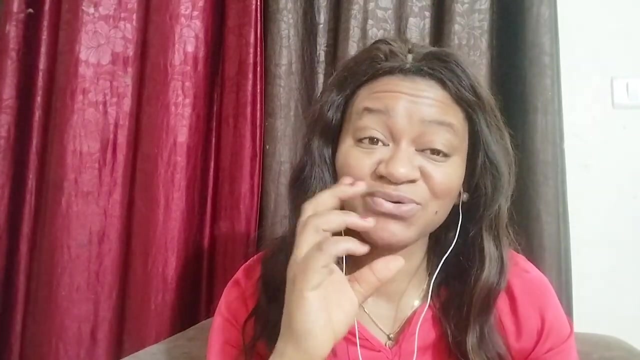 castle is located just a few minutes away from the park. I mean, this whole area is just incredible. You guys, I'm really really impressed of how beautiful- from the nature to the architecture, to everything, the buildings, everything I'm seeing on my screen right now. It's so incredible. 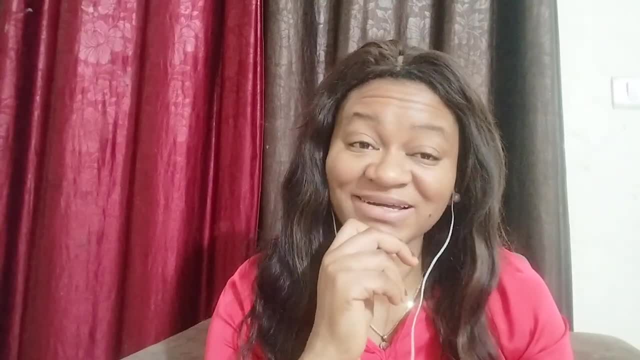 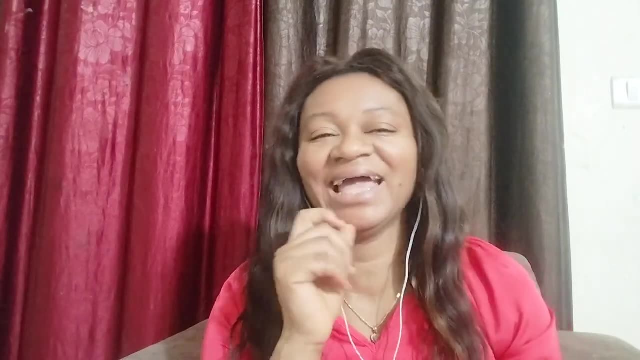 It's so amazing. This is beautiful. This is a beautiful country, guys. This is a beautiful country in Europe. I'm telling you, You guys need to visit there. It's so beautiful guys. Oh my God, Let's continue. 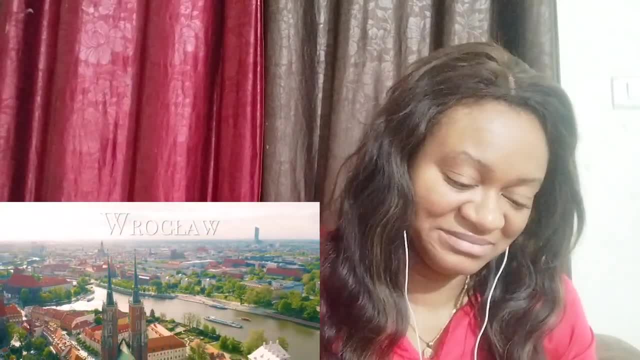 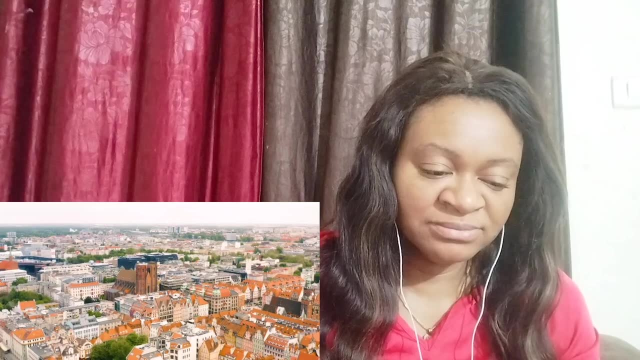 After we're going to head over to the beautiful city of Wrocław. I mean, it's such a tricky pronunciation. Now located in western Poland, about a three-hour drive from Krakow, Wrocław is such a charming historical place. It's home to one of the most beautiful market squares. 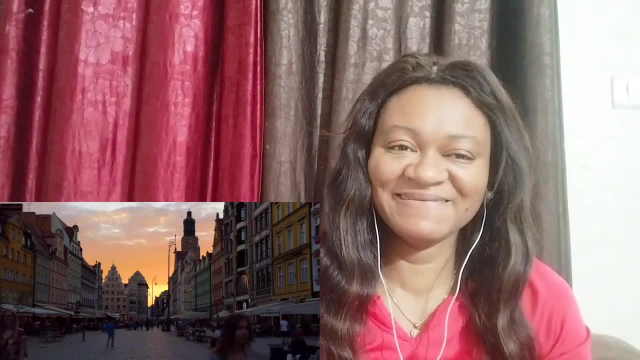 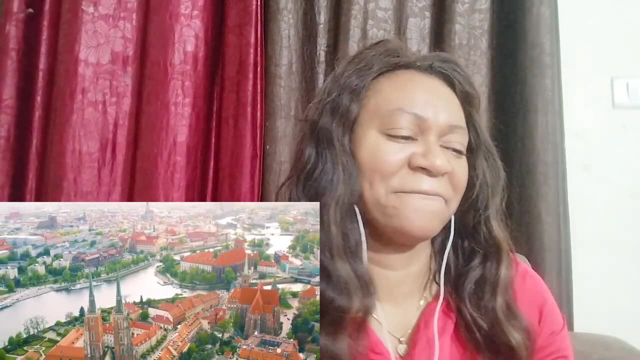 in all of Europe. Yeah, It's got townhouses and cobblestone streets. Wrocław also has one of the most beautiful cathedrals in Poland. No, It was originally built in 1272, but has been damaged and rebuilt several times throughout. 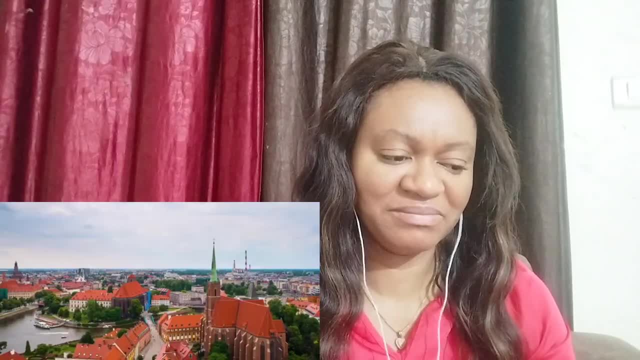 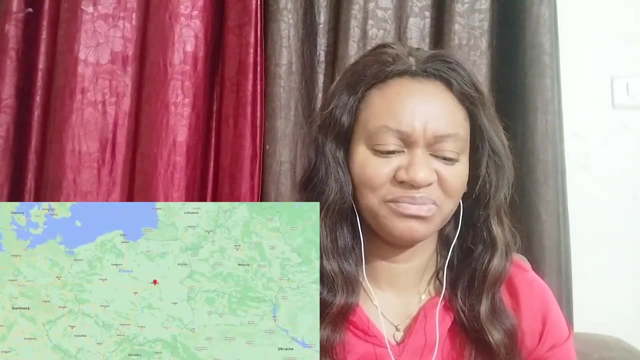 the centuries. I just love its double spires. Wrocław is just the perfect place: Just walk around and explore for a day Beautiful. Now for our final destination. we're going to head to Warsaw, located on the Vistula. River in east central Poland. Warsaw is the capital and largest city in the country. Warsaw began to grow in the 16th century when the capital was moved there. Wow, It was called the Paris of the North, but sadly Warsaw was damaged extensively during. 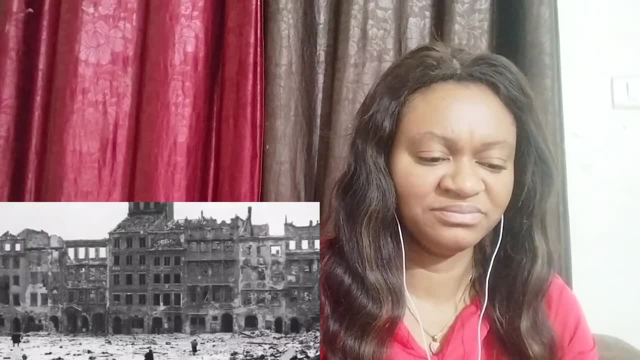 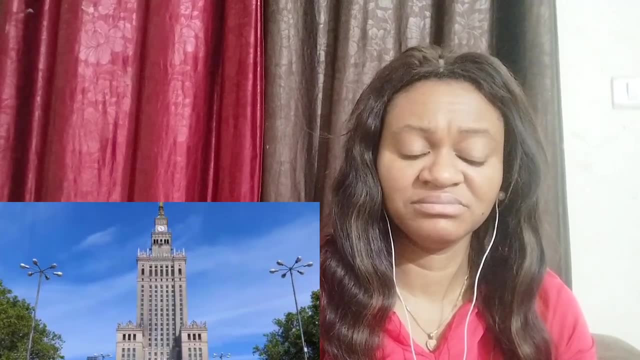 World War II, with over 85% of its buildings in ruins. Thankfully, today it's a bustling capital with a population of 1.8 million. One of my favorite buildings of the city is the Palace of Culture and Science. at 778 feet tall, It's the fifth-tallest building in the 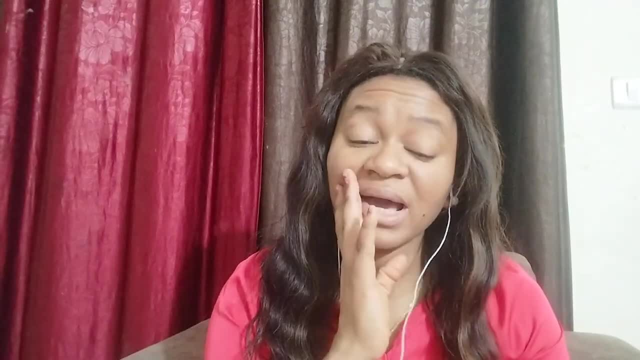 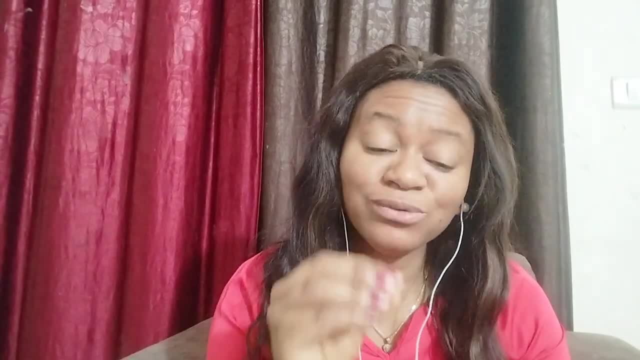 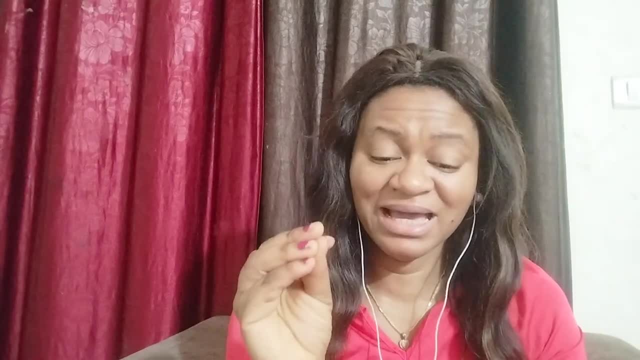 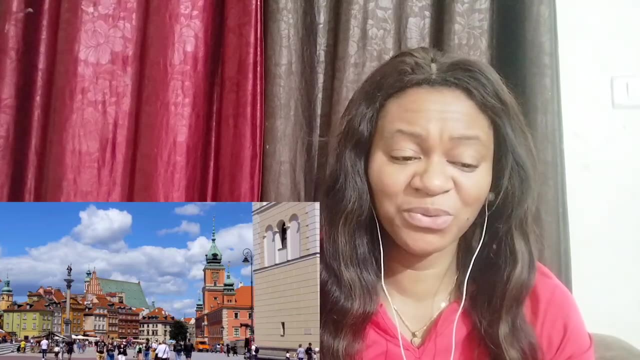 it's showing. This is so beautiful. Wow, Absolutely beautiful guys. The night views are so nice. Let's go back Warsaw's old town. it was established during the 13th century and it's full of history and medieval architecture. Like the main part of the city, the old town was almost completely. 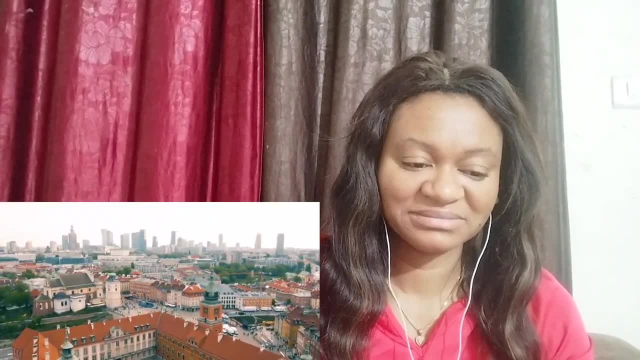 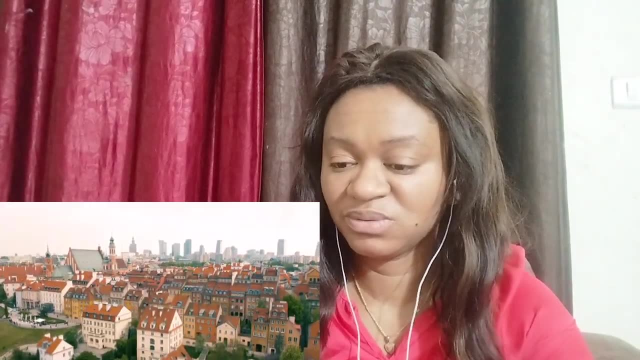 destroyed during World War II, but it was miraculously restored and was made a really heritage site in 1980.. when you're there, you can just explore the square and marvel at all the history that took place in this medieval old town. well, that is it for my poland top 10, let me know. 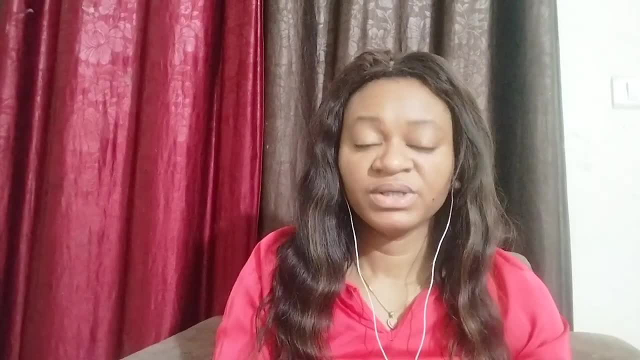 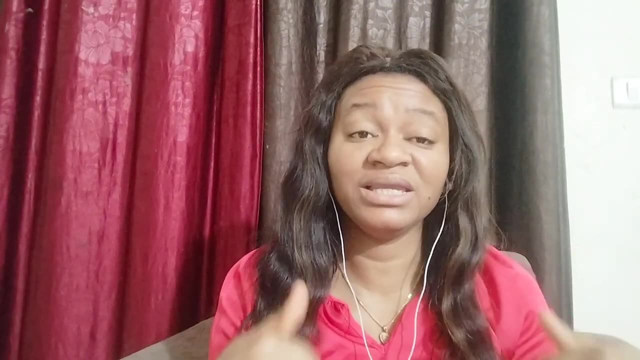 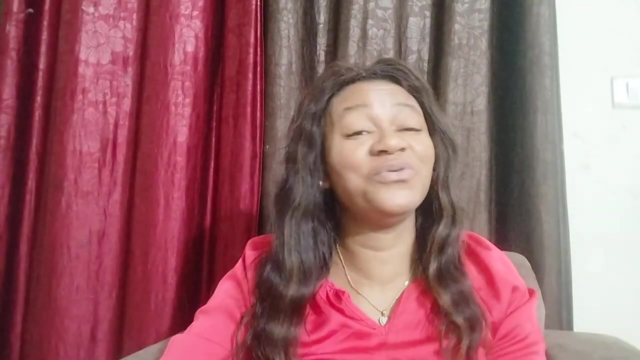 where your favorite place is in poland in the comments below. right? so you guys, i got this from ryan. thank you so much, my friend, for this. i will drop in the link in the description box below for non-interrupt watching. okay, thank you so much. i love, love, love, love poland. we've seen these also. 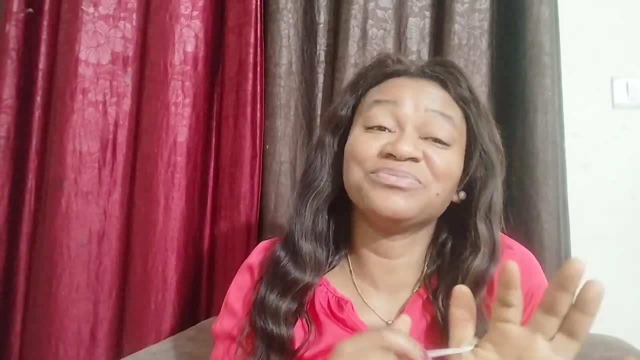 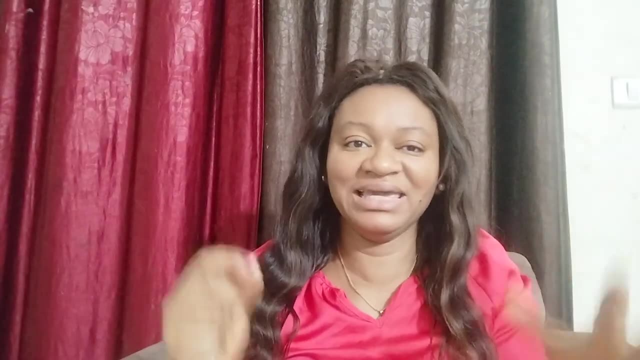 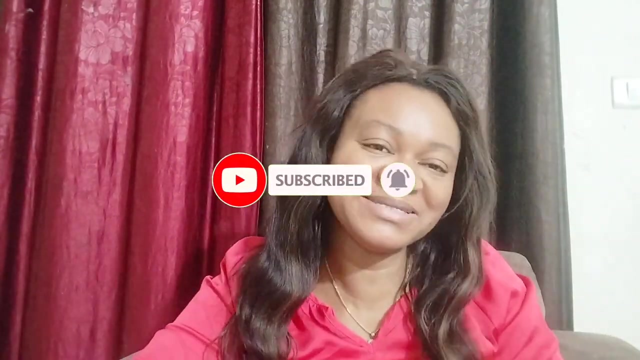 increase my desire to visit there. that was a beautiful, that's a beautiful country, unique country after all the destructions, and they stand back again. thank you guys so much for watching. i hope you enjoy watching. please don't forget to subscribe to my channel. don't forget to like. i'll see you guys in my next one. peace out. 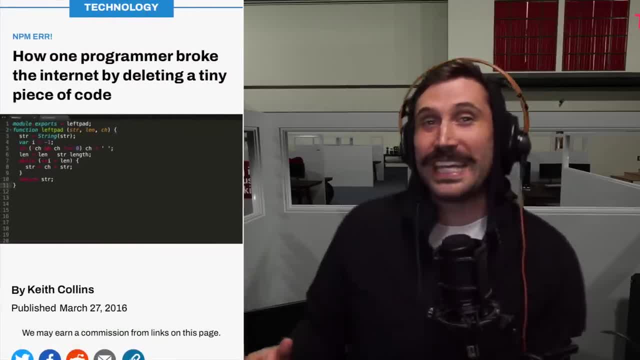 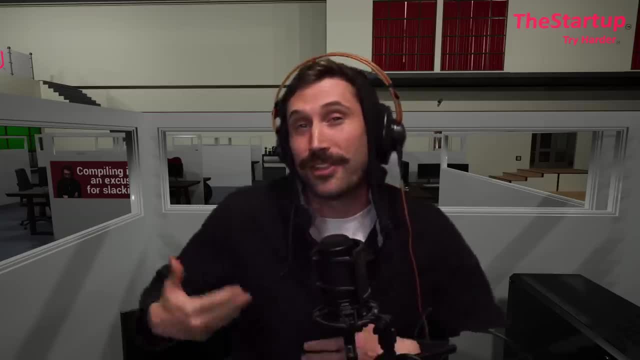 LeftPad, an 11-line piece of code, broke the internet and just recently had a second incident that involves me, So I might have made a mistake where I thought I could program a faster version of LeftPad live And the results were not faster. 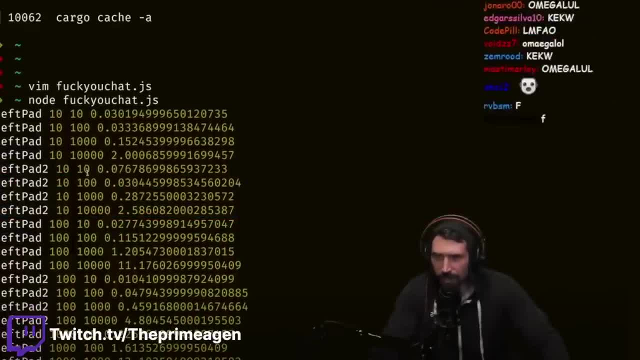 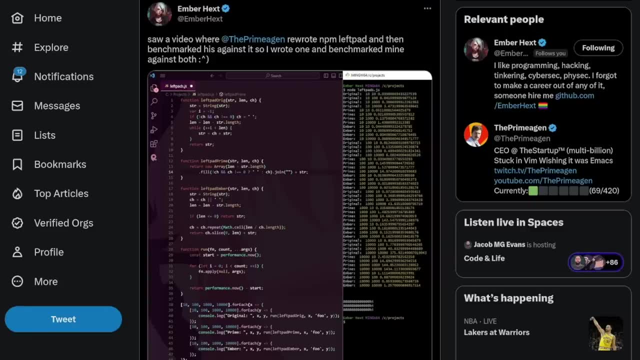 It goes to here LeftPad with this one. Okay, so it looks like mine is slower. Oof, you hate to see it. At first it inspired a meme. Then Ember Hex made an actually fast version. Then the creator of Crab Lang threw his hat in the ring. 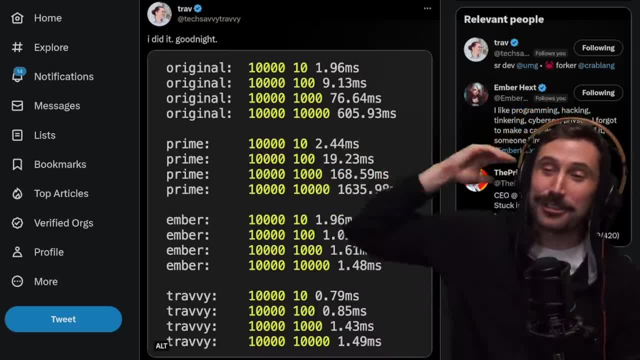 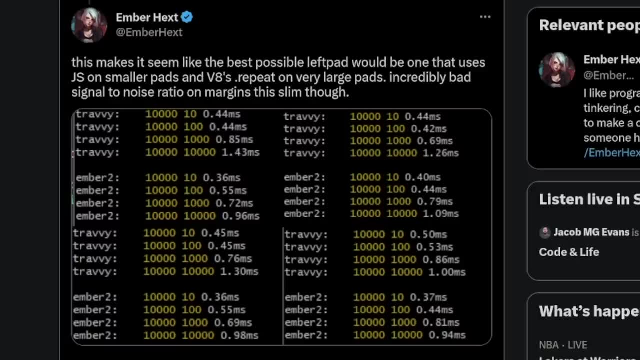 Even faster than Ember's, and mine is still so slow. A renaissance of LeftPad happened, and other people were joining in, And then a competition was born: Who had the fastest LeftPad? Submissions were made, More submissions were made. 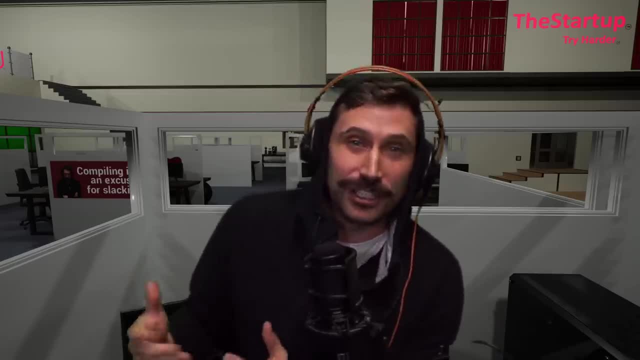 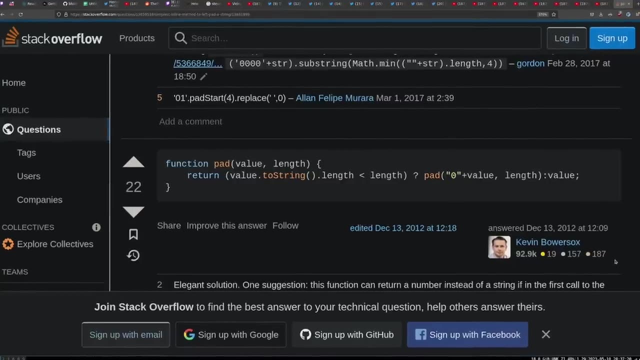 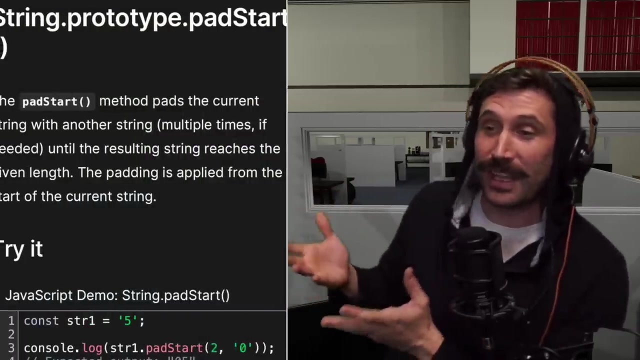 Then corrected, And meanwhile I was hating life on YouTube. I'm officially cured of imposter syndrome. Oof too spicy. Even Stack Overflow had their own bespoke solution, and it was recursive. Not only that, but there's also a native LeftPad solution provided in modern JavaScript. 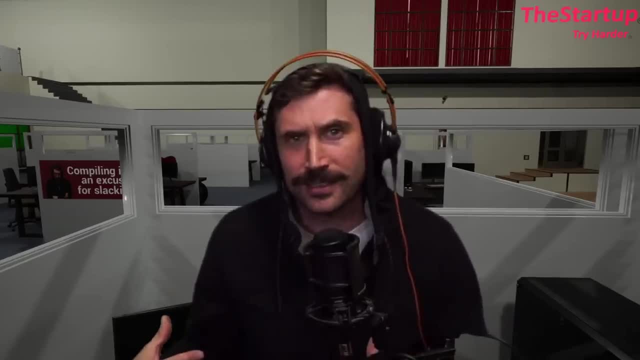 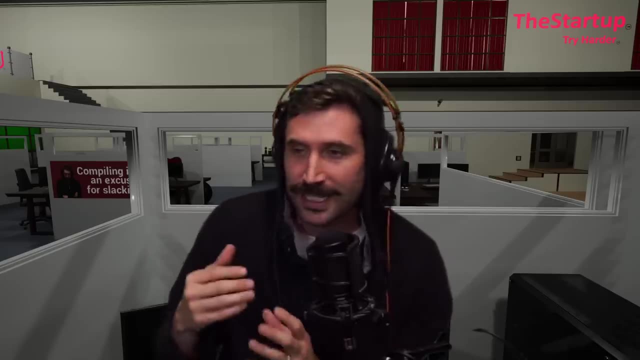 And we need to figure out which LeftPad is the fastest And find out. do micro benchmarks lie? Yes, they do. So this competition has been about micro benchmarks, But here's the thing is that some of you might not even know what micro benchmarks are. 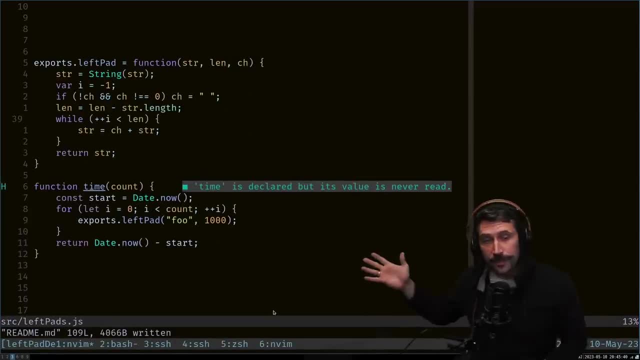 Well, they're as simple as this. You write a function you wish to test. You run it a bunch of times, taking a bunch of time. You run different differentials and you see which function performs better than the other. You have different implementations and you hope one of them is going to perform way faster. 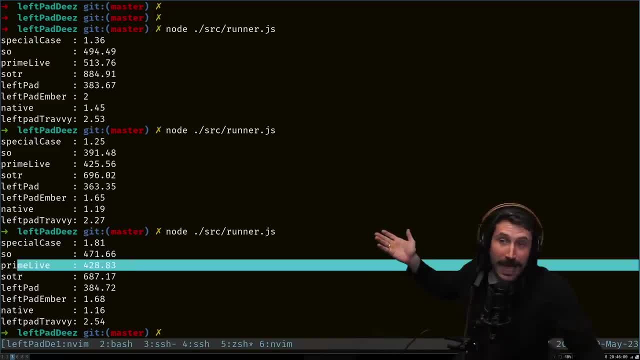 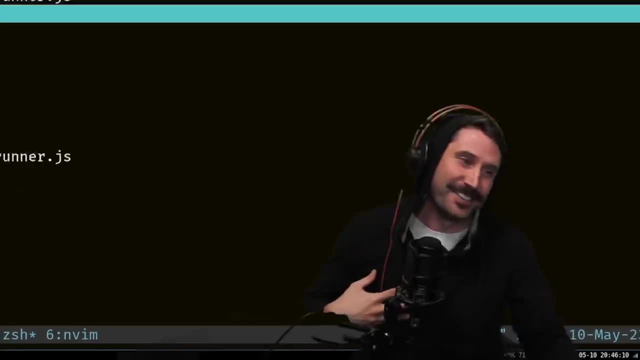 Then you run it a whole bunch and you see that some of them are much slower- Say mine or the Stack Overflow one- And some of them are way faster, like Ember's or the native one, or the special case one that I also have in a right.